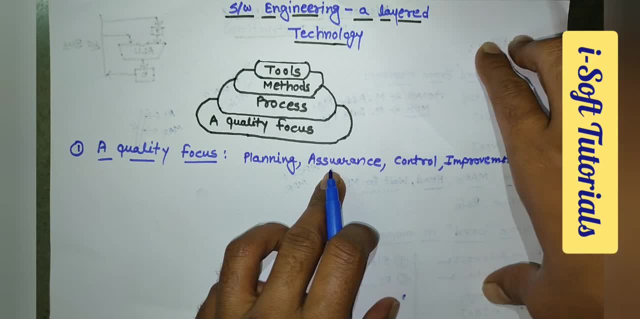 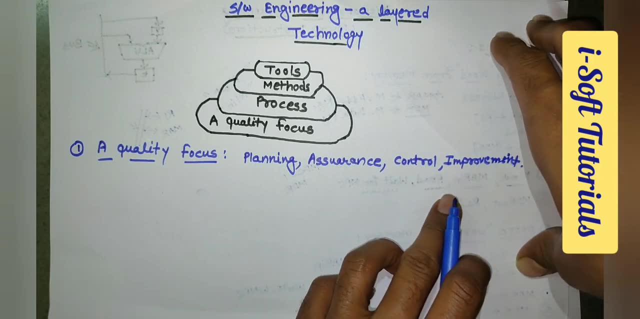 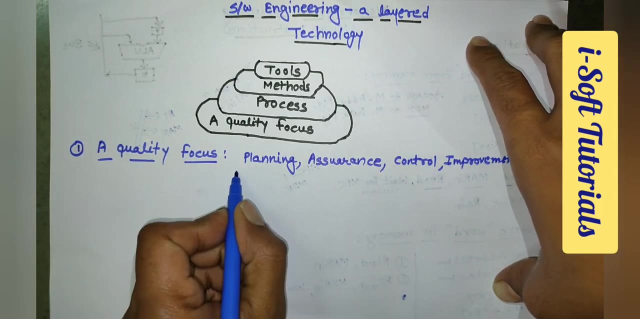 to consider proper planning. We have to assure, assure that what we will develop, that is correct. Then we have to control overall process and also we have to focus on improvements. So hence it act as a base layer or a bedrock, So it can be considered as bedrock layer, Then after focus on quality. 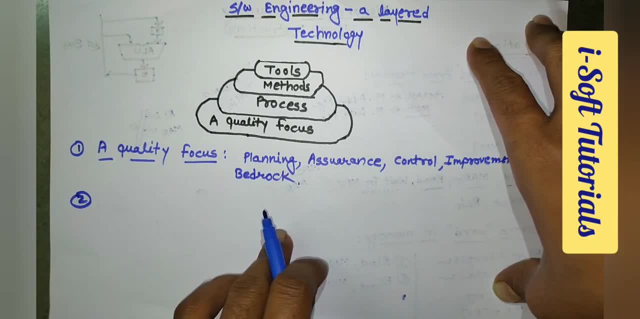 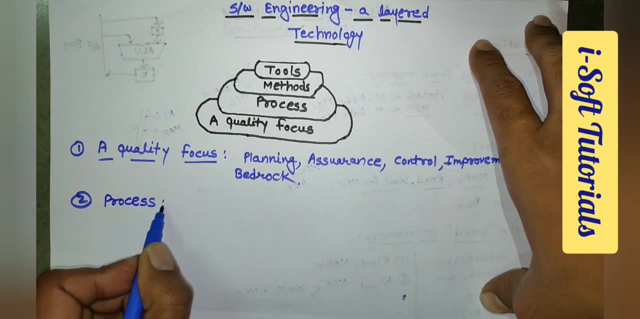 after clearing all the requirements, then after proper planning, after assurity that we can develop the software, after considering control measurement, now we can proceed for process. so process layer. So what is process layer? Process layer is Foundation and glue of software engineering. 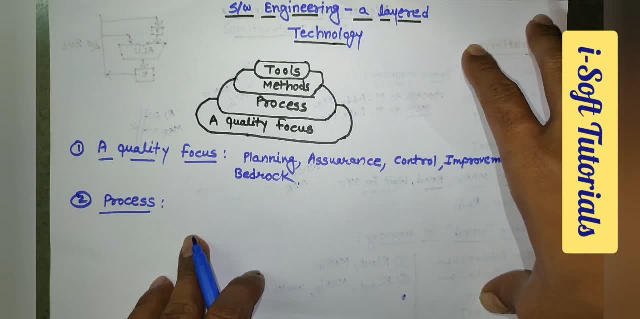 Why it is called as foundation or glue of software engineering. It provides structural support for software engineering. It defines a framework for effective delivery. It provides structural support for software engineering. Here we have to provide proper engineering. honestly, it is a framework for effective delivery. to make it quote-unquote: ok, exactly, It provides. 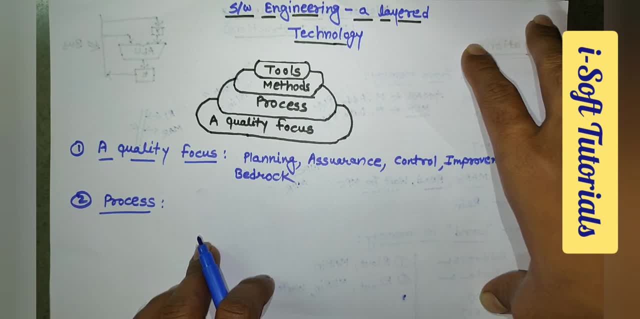 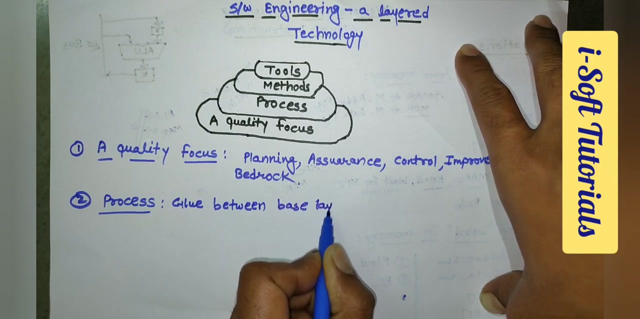 means all the structures or all the architecture of soft training engineering process is decided in this process layer or next step or next layer. so this is acting as a glue between the base layer and it is acting as a glue between base layer and implementation or methods and tools implementation. 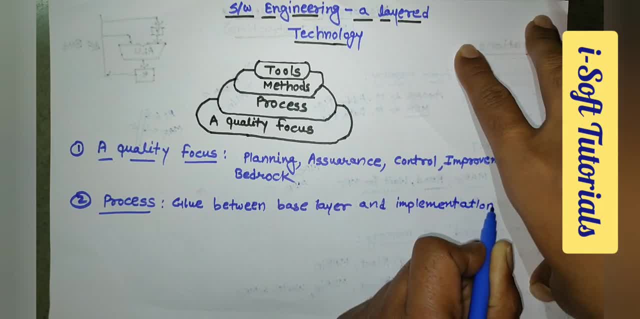 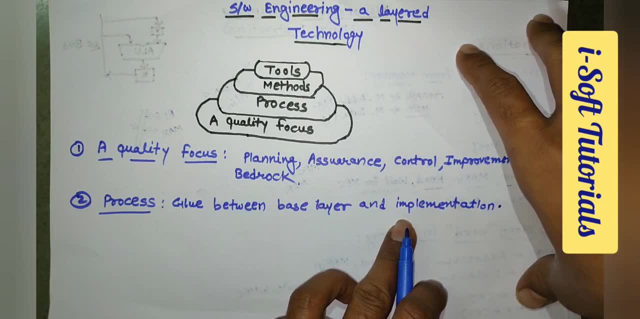 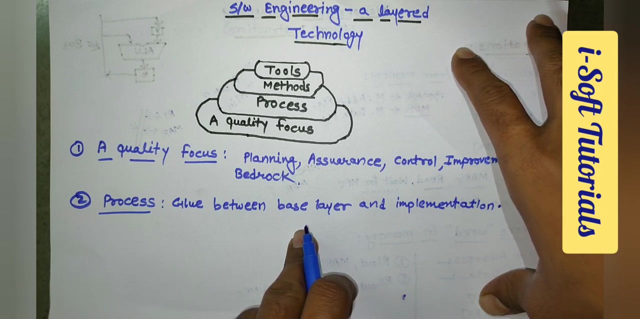 layer, that is, methods and tool. so it is acting as a glue between base layer and implementation may, or methods and tools layer, and it is also deciding all the architectural part of software engineering process means how the software engineering engineering process will be performed. then what are the models that we will use? what are the methods that we will follow all this part? 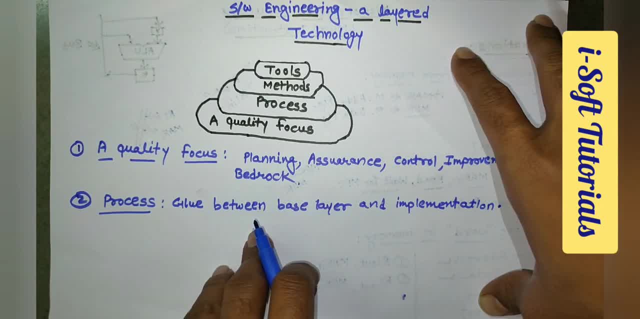 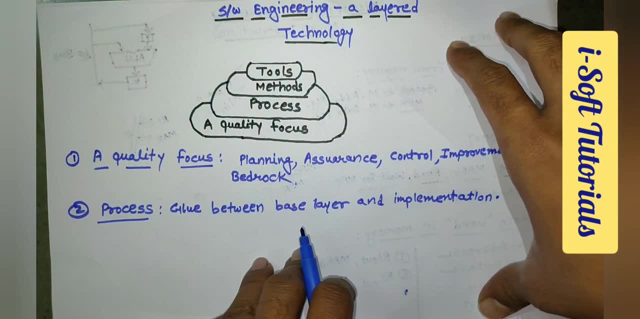 are included in this process layer, then it act as a blueprint and provides basic management, control or overall, the overall process or overall process. what it provides, it provides meaning to the product. that means it also decides what is the work product or software product that we are going. 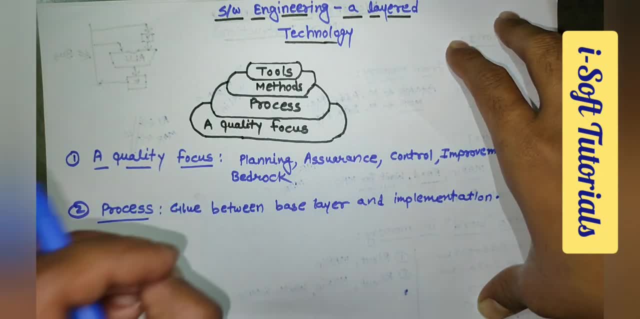 to develop? what are methods? the method that we are going to use, that we are going to use in this, that we will apply. what is the quality of software that we will develop? all documentation part is included in this step then, like, for example, SRS or design documents or reports. 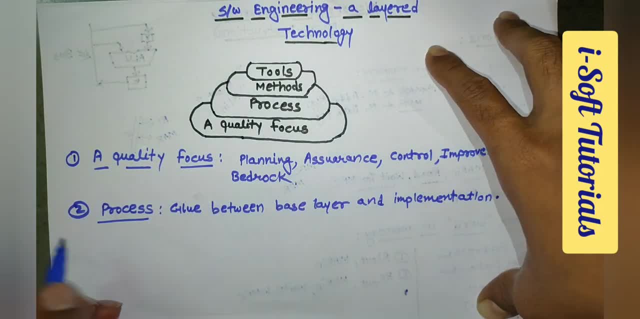 that are created in this process layer after creating this architecture part of software engineering. architecture part means after deciding how we will proceed. then we can proceed with methods that we have selected in process layer. so what this methods layer provide? it provide technical meaning of software engineering or technical methods of software engineering. 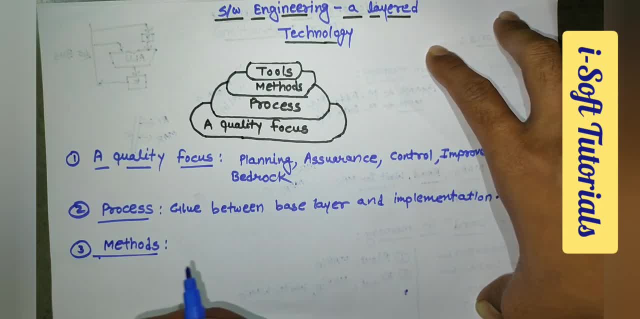 that we will use for software engineering is pro. it provides how to develop or how to build the software. metal methods will include requirement analysis, then design, program program construction. it includes testing and also it includes support. so it includes methods of development of software, methods of for development of software. that means models, then technologies, then program construction. 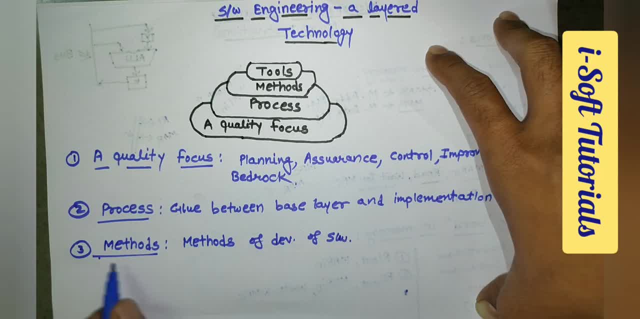 then design of program testing support. all these things are included in this third layer. then fourth layer is tools. so these tools, whatever methods we have selected for that, what tools are required that are included in this layer? it, the software engineering tool- provides automated, semi automated support for the process and the methods, whatever process we have selected, whatever methods, models we 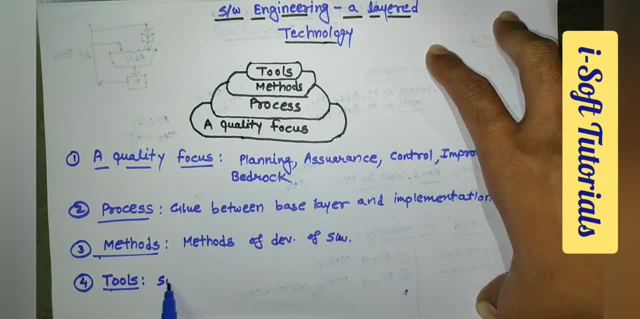 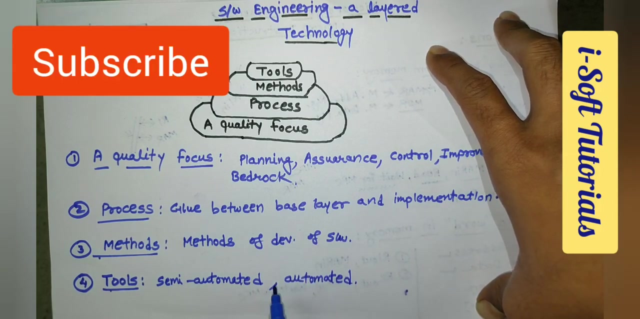 have selected for that. whatever tools are required, that tools, that is, semi automated or automated tools- are included in this layer. so this is the soft engineering as a layer technology, layer by layer, we have discussed. if you have any doubt, please comment in comment section. please like this video, share this video with your friend and subscribe to my channel. thank you.